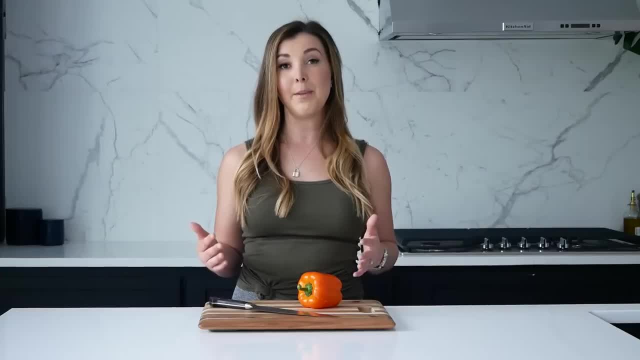 Of course, I've grown my collection and got different types along the way, but I went to Williams-Sonoma and I just looked at all the knives. I didn't know where to start, and the best advice I got from some of the chefs that I first started working with was get what feels good in. 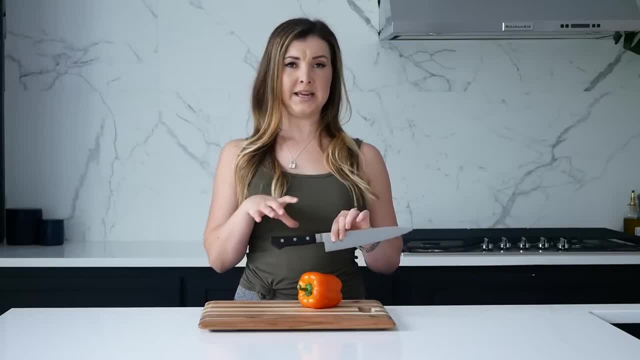 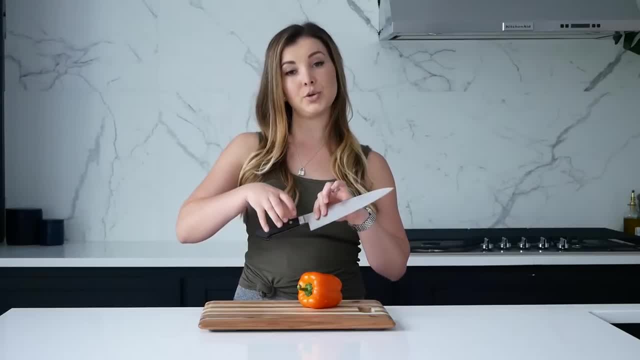 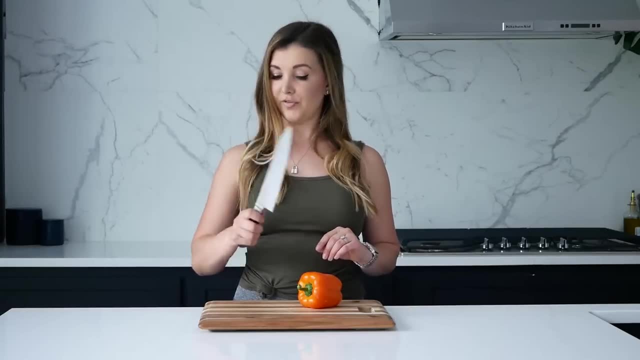 your hand. I personally like a little bit of a thinner grip. Some of those bigger grips just make me concentrate on my grip too much. I just like something that just kind of easily fits in your hand. The very first thing that people like to do is put their finger right. here. I did it at. 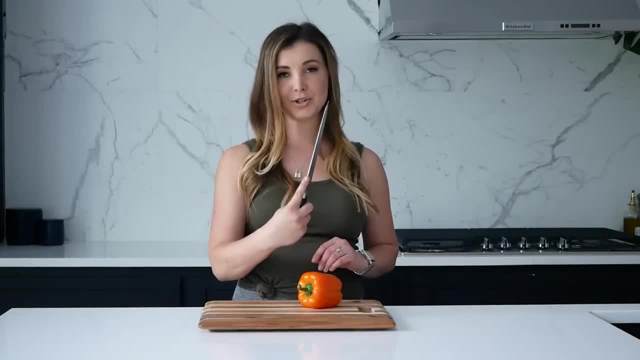 the beginning and people were like: no, no, no, no, That's not how you do this. Do not put your finger here. You're going to just kind of rest the knife in your hand, lightly grip it, You don't want. 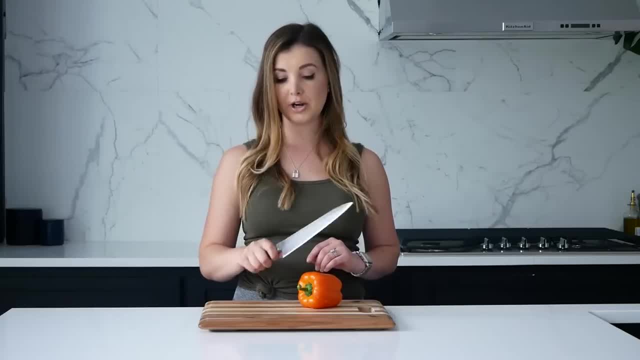 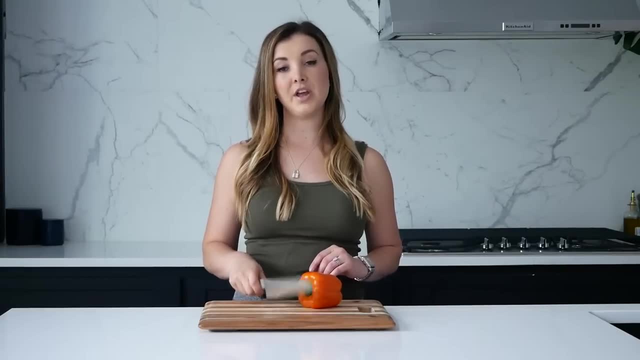 to squeeze it, but you don't want it too loose or it's going to fall around. Just firmly grip all of your fingers, Just kind of tie it like that in a knot, and that way you have complete control over the knife. The thing about the blade: so they come in all different shapes and sizes. Just start with a. 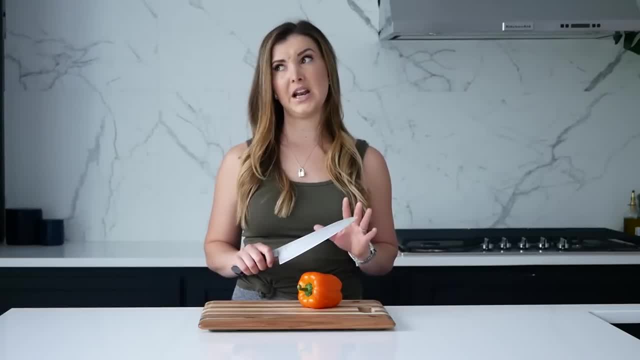 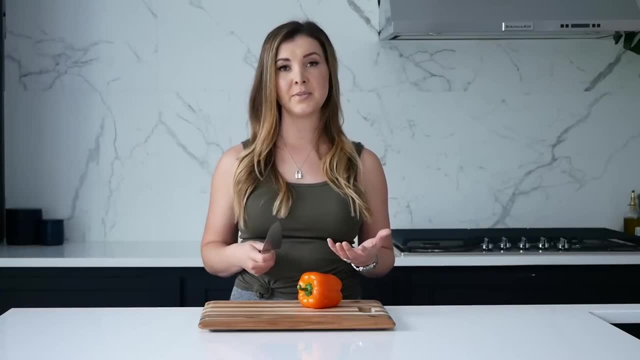 basic chef's knife. The bigger the chef's knife they can get upwards. I think of like a 12 inch chef's knife. That's actually pretty big. I think mine are typically 10 inches. I think that that's just a good size for me. Again, if you're a big guy with big hands, then maybe that's something. 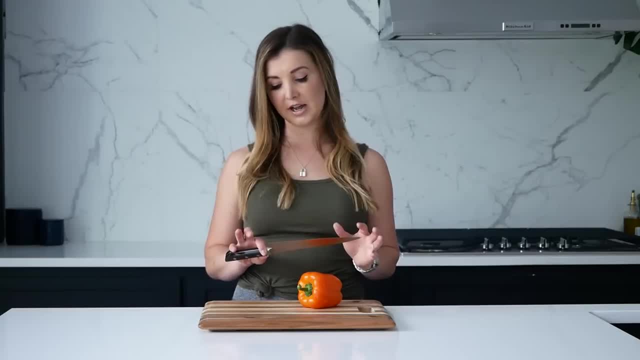 that you feel comfortable getting into. I like the 10 inch chef's knife. So again, just kind of tie it like that in a knot, and that way you have complete control over the knife. Just kind of tie it like that in a knot, and that way you have complete control over the knife. 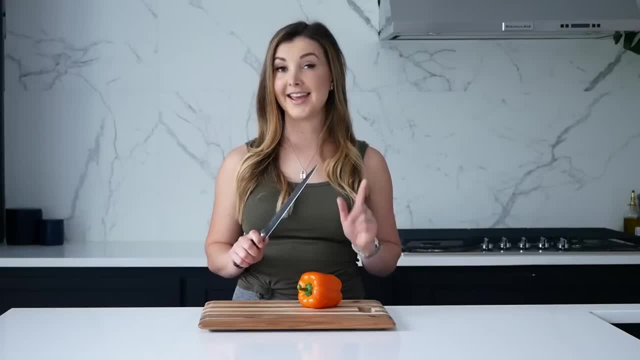 Just something simple, something that feels good in your hand. And then the other main point is: make sure it's sharp. I will do a whole other video on how to properly sharpen your knives, but typically right out the gate your knives should come pretty sharp And most stores that. 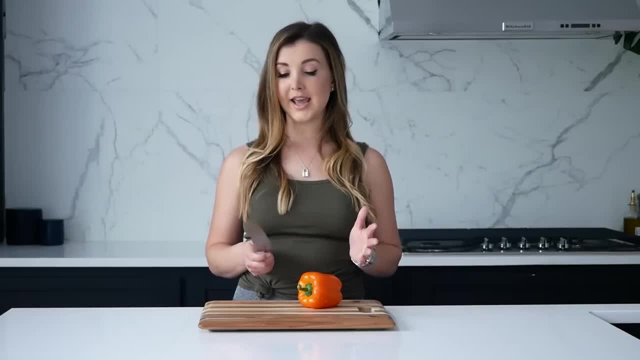 you can purchase them, for you can actually get them sharpened there Or again. I'll have a video for you guys here shortly on how to properly sharpen your knife. So first thing that we're going to get started is not even diving right into a vegetable, We're just going to start right. 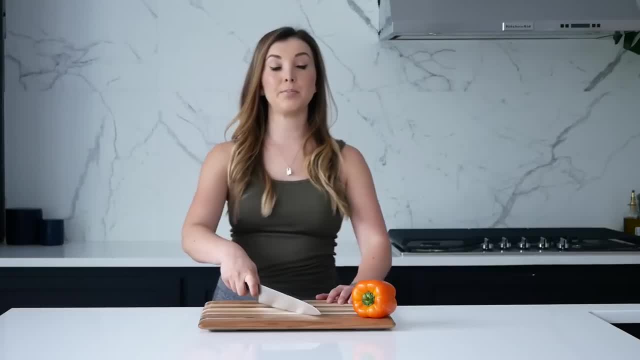 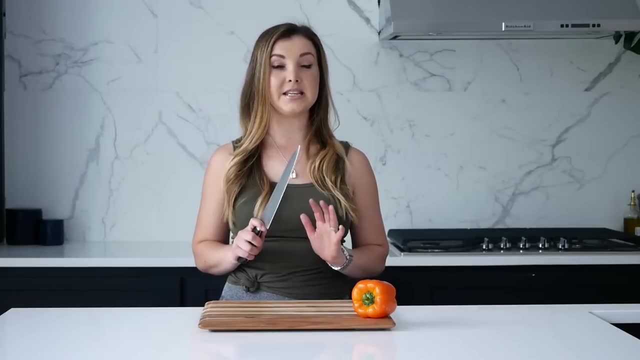 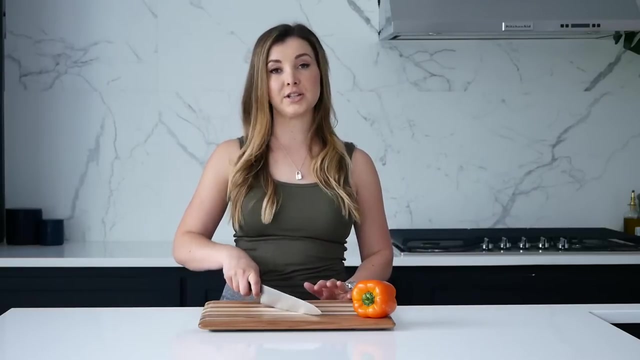 here on our cutting board. This is kind of how I learned A lot of people want to jump into just like chopping super fast. You got to start slow, I promise, I promise, I promise The speed and accuracy will come with time. It is all about practice. So, first things first is you're just 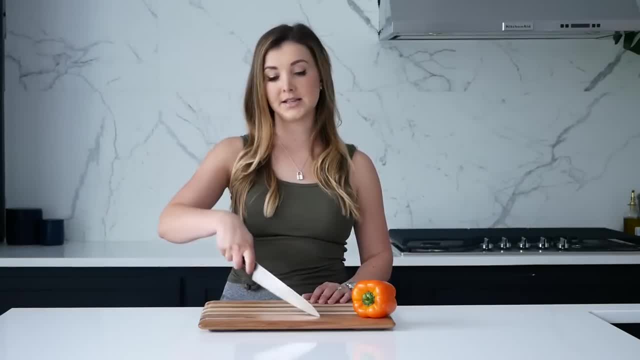 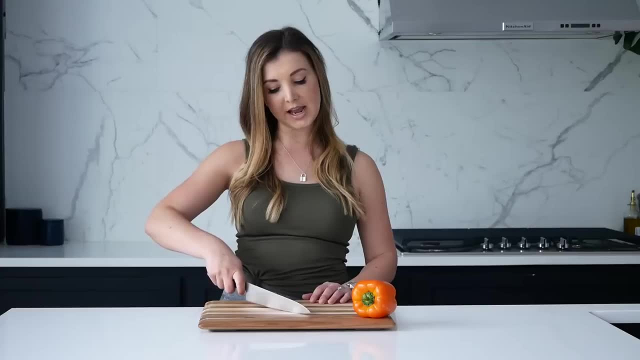 going to kind of gently rest the knife on the board and you're going to practice a rocking motion, kind of like a boat. So the tip is going to be kind of like pointed down, You're going to push down and up, So again, 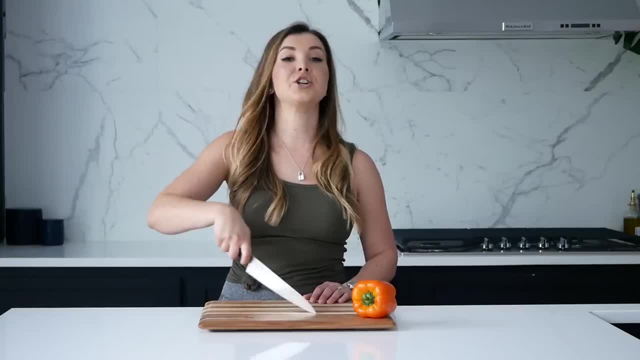 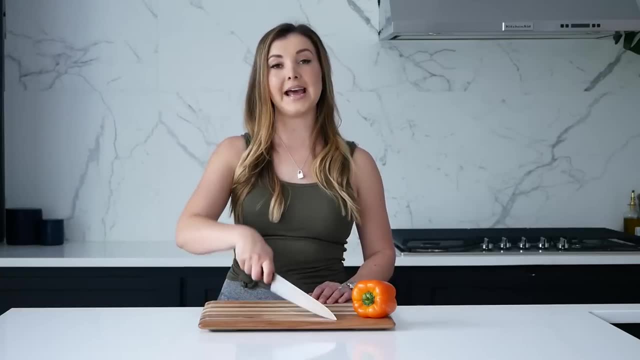 kind of a rocking motion with your hand and at the board and just sit there and get comfortable. Don't chop anything. Just slice your board and get this really rocking motion And that is how you're going to cut things. You're not going to just press down into them. That smashes the 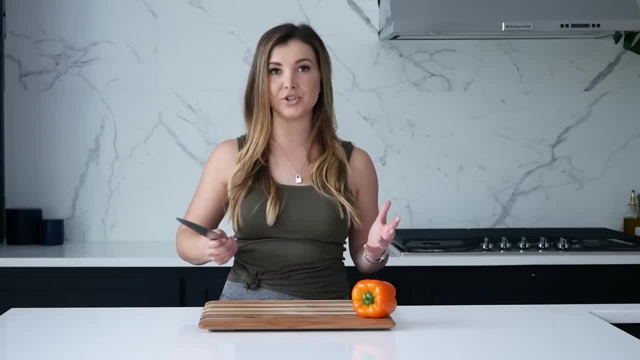 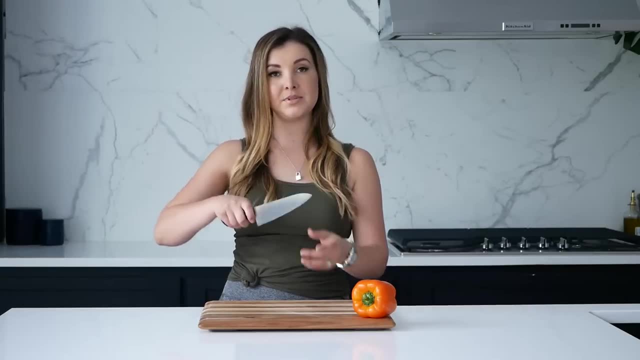 vegetable does not slice the vegetable or whatever else you're cooking. So especially this is going to kind of guide the knife on it being sharp all the way through. A lot of times if you just use the middle of the knife, that'll get dull and you'll have to use kind of the. 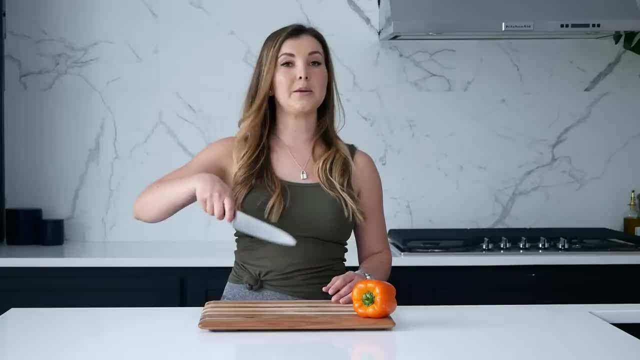 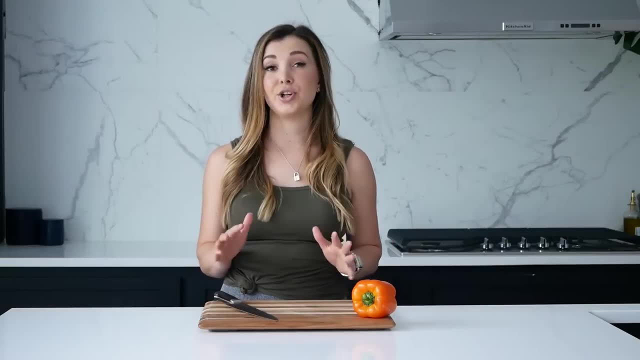 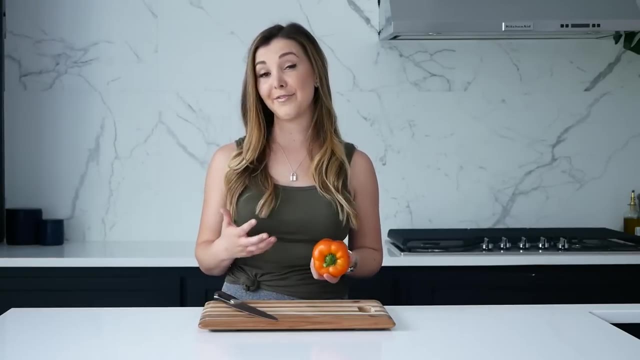 tip or the back part of your knife to get that sharpness. This just keep it consistent front down and rock the boat like that. So the very first vegetable that I ever learned how to properly cut and dice and slice is a bell pepper. Chef Kent Rathbun was the very first chef that I ever 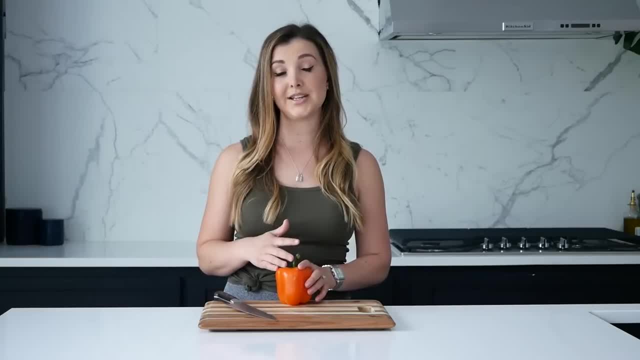 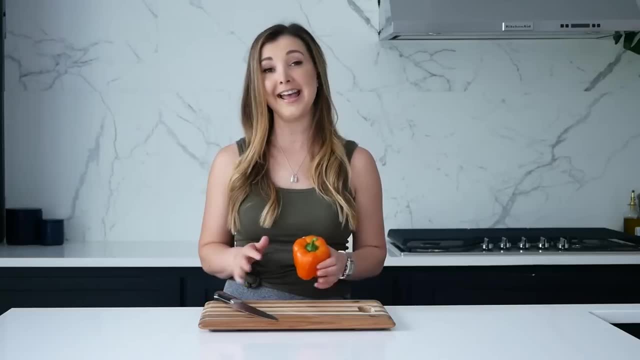 worked for And I had moved from Austin to Dallas to work at his restaurant, Abacus. I started out just doing prep, had no idea what I was doing. Can't believe that. let me in the door and work there, But I learned so much. 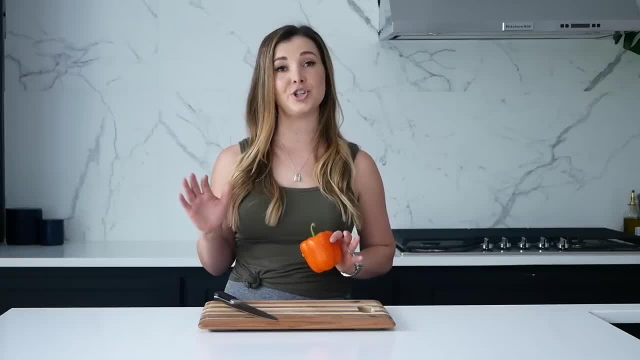 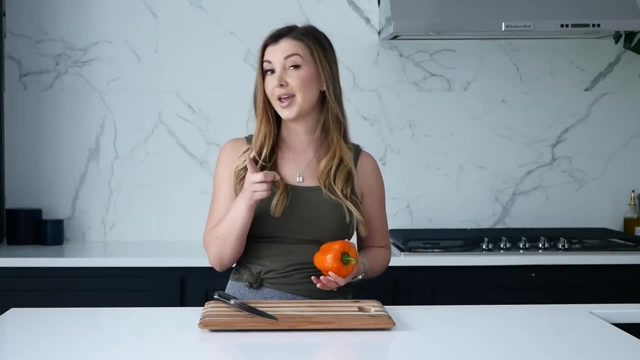 And him and his wife Tracy were super kind and just brought me under their wing and wanted to teach me everything they knew, because they knew I hadn't gone to culinary school. That's another thing. It's okay, You don't have to have a proper culinary education. I still 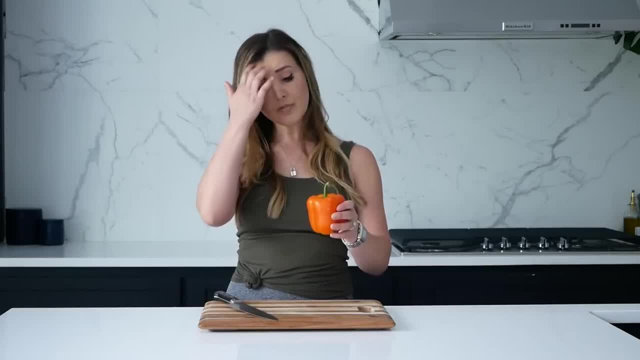 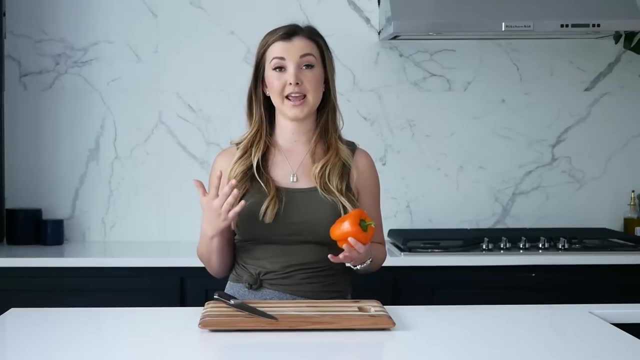 to this day have never taken a culinary course. So they brought me into their house one day and was like: listen, we have an event, We're just going to let you chop our vegetables and get some practice. So they showed me very first how to chop a bell pepper. So I thought 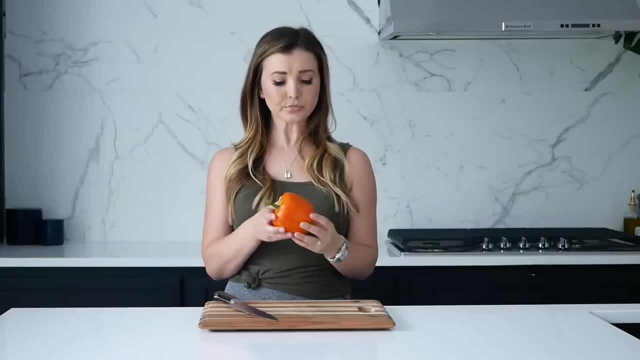 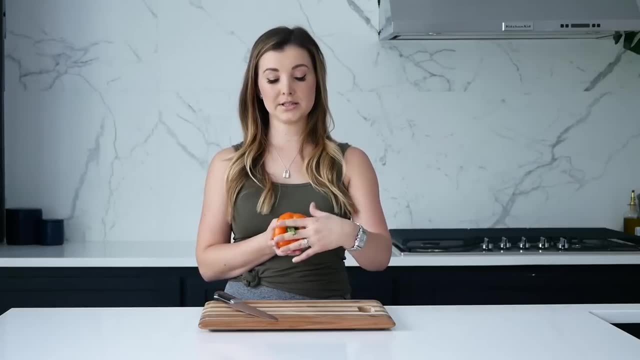 I learned that first. I'm going to teach you that first. So a bell pepper, a little bit different than chopping an onion, but this technique can actually be used on a lot of other vegetables as well. So the vegetable, this bell pepper, has the stem end and kind of this end over here. So the 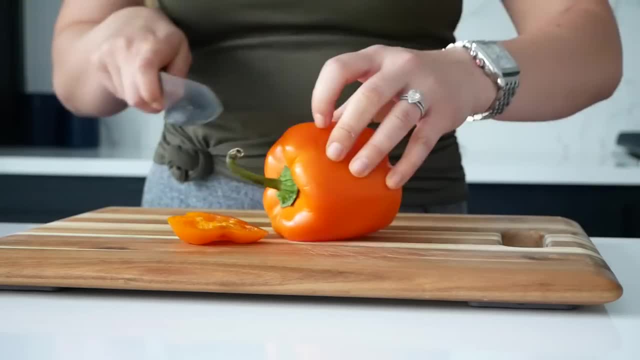 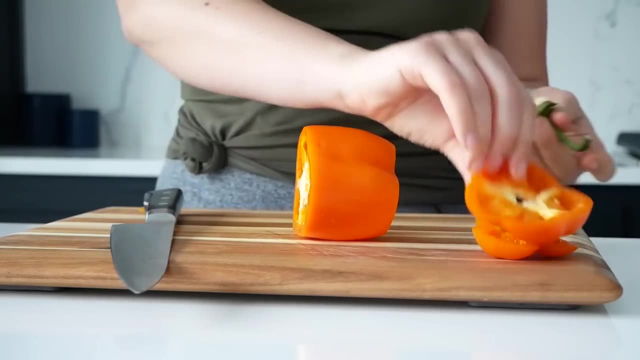 very first thing is you're going to just slice off the ends, And you don't want to slice off too much, especially on the stem end. You can kind of get a little resistance from the stem, That's okay, And then you're going to pop the stem out. These, however, can totally be used, So do not. 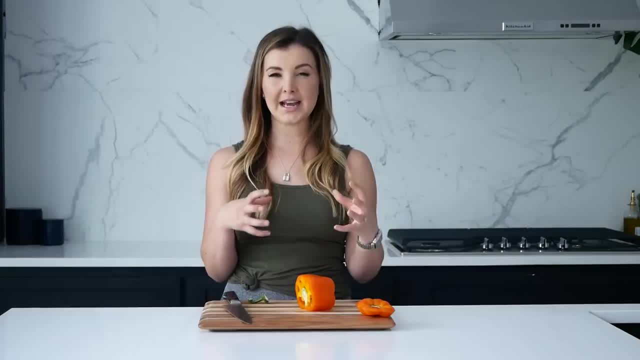 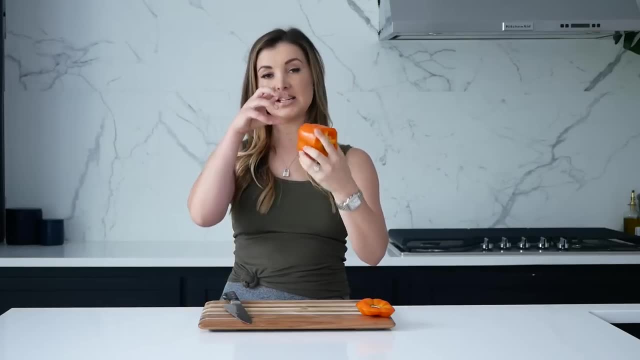 throw them away. Just set them aside, Cause I'm going to show you how to get a nice clean cut. So toss that, and you'll have the middle of the bell pepper. So instead of just digging your hands in here and grabbing this out, and then you're left with kind of these, um, these little grooves in, 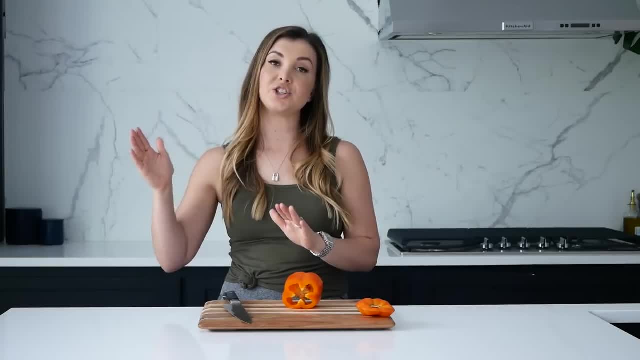 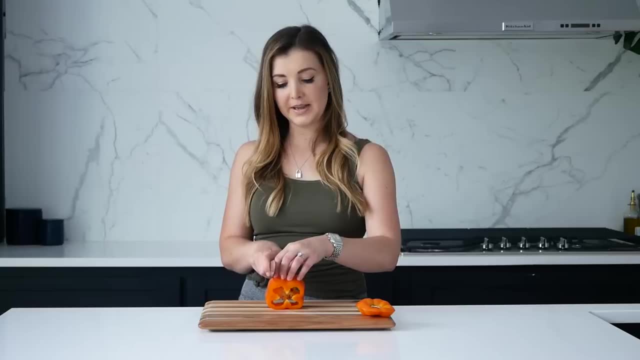 the bell pepper. you're going to slice it And you're basically- the technique is called flattening out a bell pepper- So you're going to start and get the bell pepper nice and flat And then you're just going to pick a side that you feel comfortable and kind. 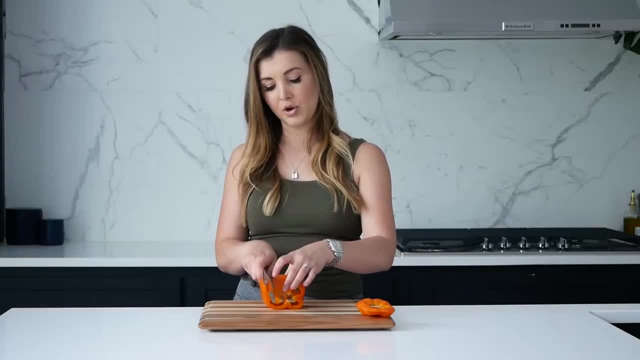 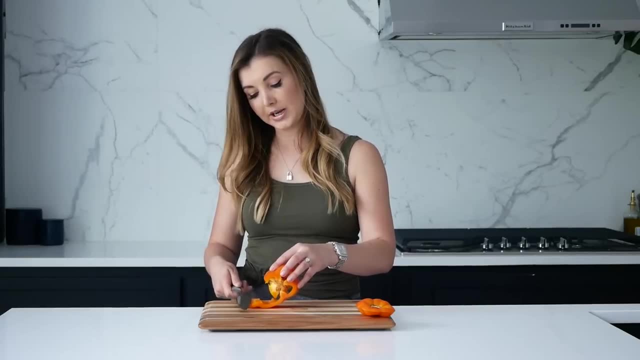 of get your fingers up here And you're just going to start to make a slice. Now you're kind of like opening up this bell pepper. So then here, take this slice that you've sliced. You can kind of hold this other part here. You're going to press your knife down like give it some weight. 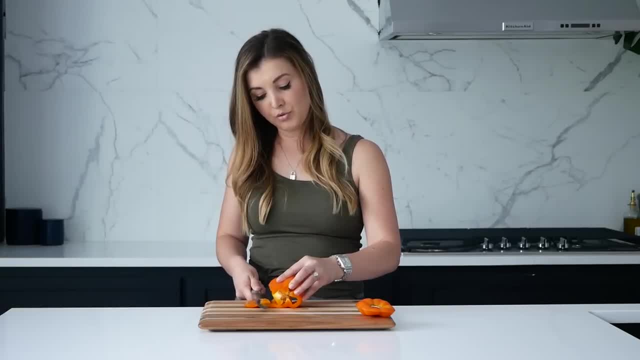 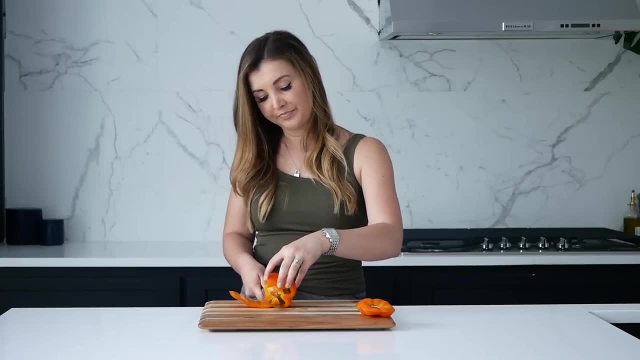 to it And you're just going to start to kind of move the knife just equally as flat. We're not getting, we're not. we want to keep it super straight and just press down and then kind of pull back the bell pepper as you get to the next part. 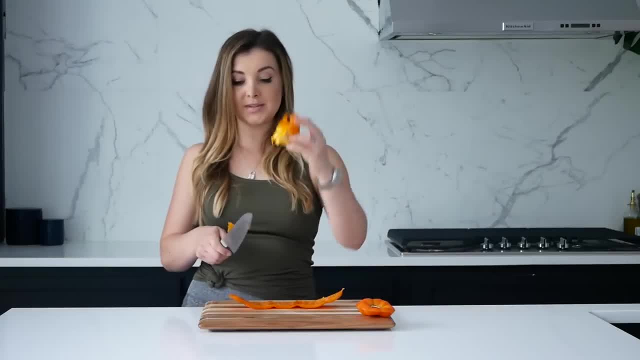 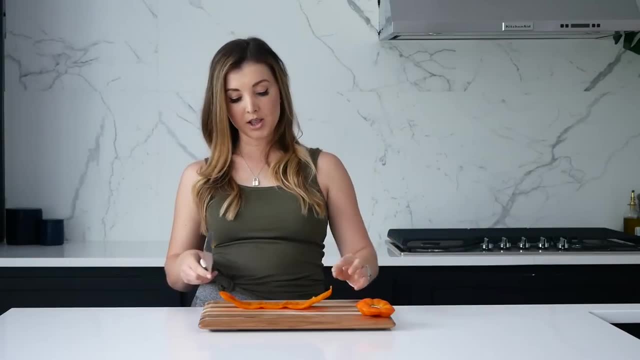 Boom, This all comes out. You do not use this, so we can just go ahead and toss it. So now, this is what we're left with: the bell pepper. Now a lot of people, for most people at home. you do not need. 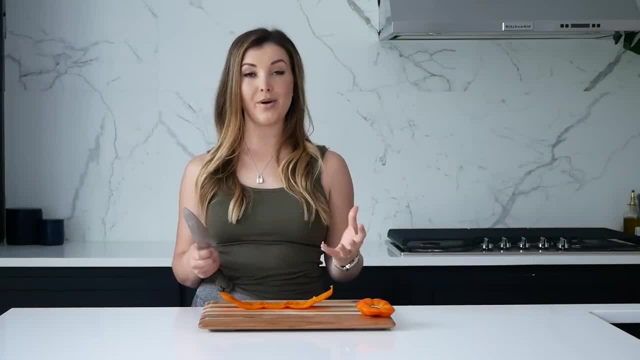 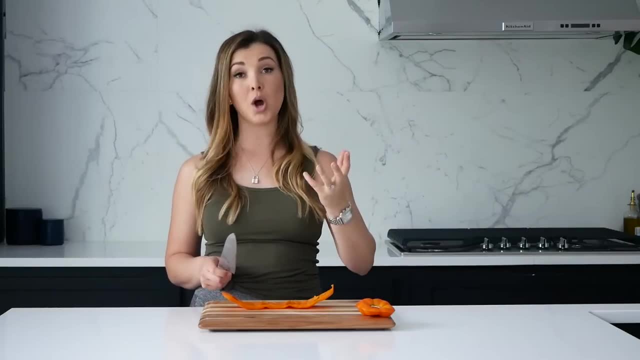 to get crazy and kind of shave this down more. Uh, these will be great. However, in kitchens we like it to be super, um, precise, And especially when you're trying to get a teeny, teeny, tiny dice like a brunoise, you will continue to actually kind of shave off some of this extra skin. 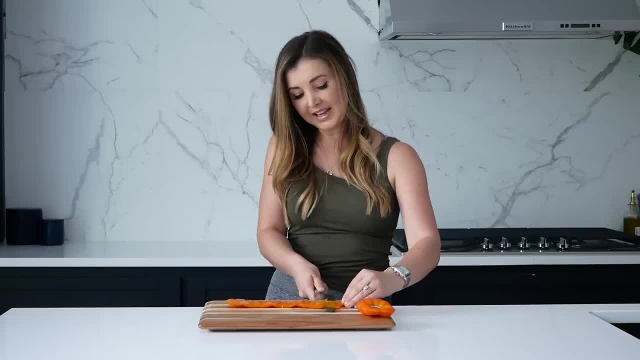 And again, you don't have to do that, But you're going to want to do that, And then you're going to have to do this. but I'm just purely showing you this And it's just nice to practice for your knife. 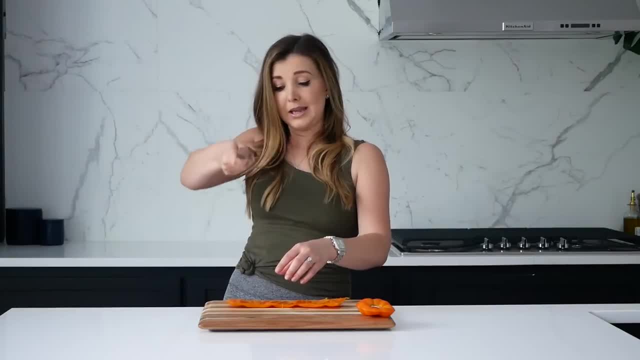 skills. When I first started doing this, my knife would be like: ee, ee, ee, I would like chop into the pepper, chop up and chop. It was a hot mess, But guess what, It's okay If you're cooking at. 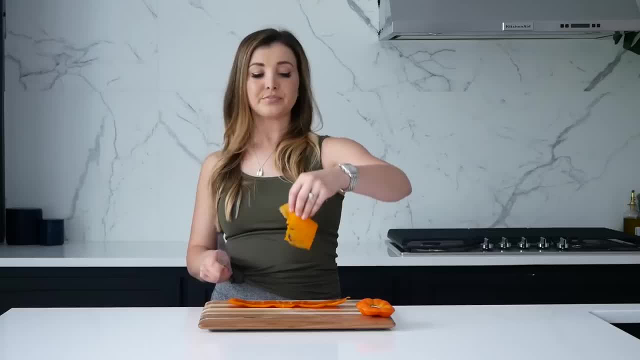 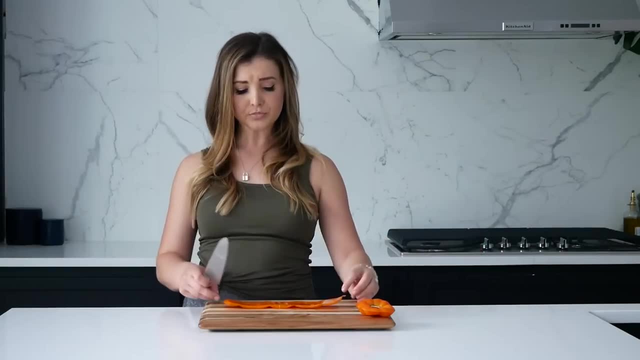 home. no one cares what it looks like. You're not in a restaurant. So again, you can chop this up, put it in salad, or today, I'm just going to toss it to the side, put it in my compost bin. So as you. 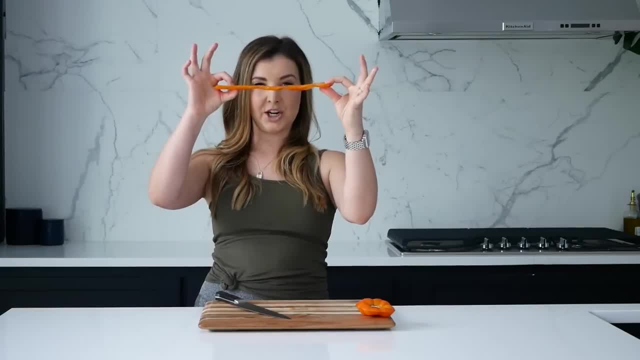 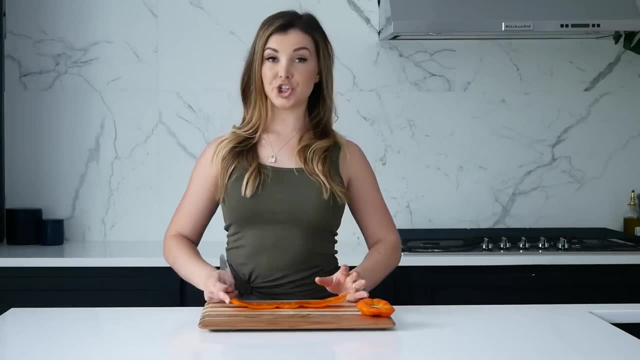 can see now it kind of has a little bit smoother texture. It's a little bit thinner and more even around. Again, you don't have to start that, but I figured I might as well show you how to do that. So when I chop vegetables, you want to make them or cut them into manageable pieces. So 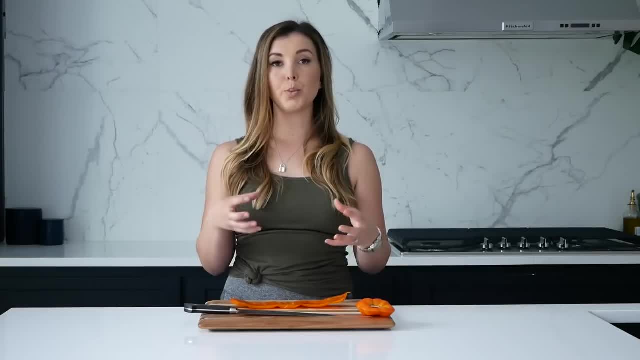 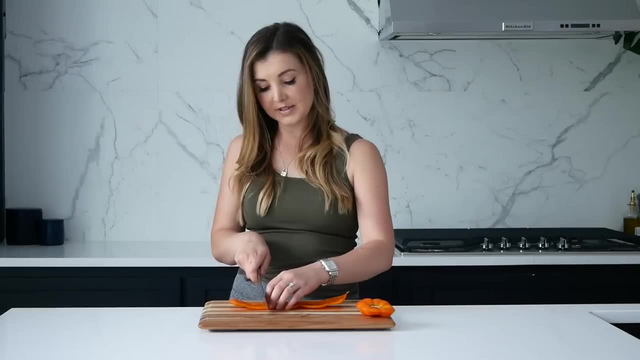 everyone tries to tackle, like these giant onions or these giant peppers, break them down to the size that you feel comfortable working with. So for me there's. I don't need to kind of chop all of this at once, So I kind of divide it up in two thirds. So have these pieces Now here. 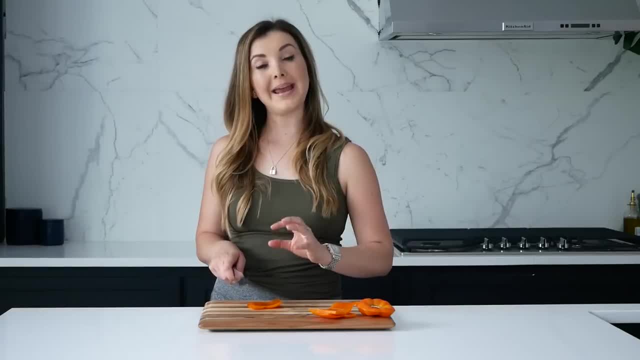 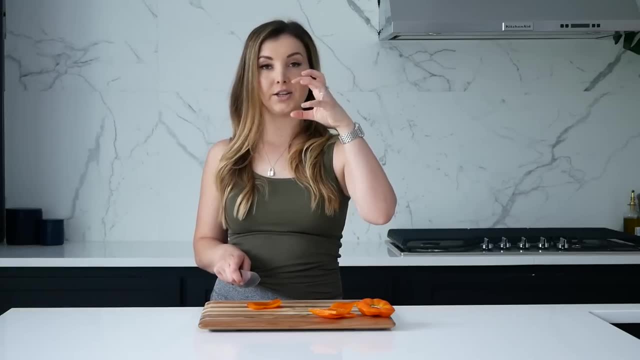 you will then start to work with it. So when you grab anything um with when you're about to die, slice whatever you want to practice the claw technique. I know this looks a little like overbearing. I know when you look at chefs on TV they're probably not doing this crazy claw. 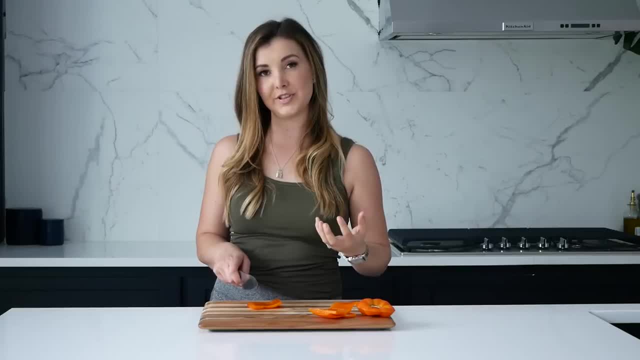 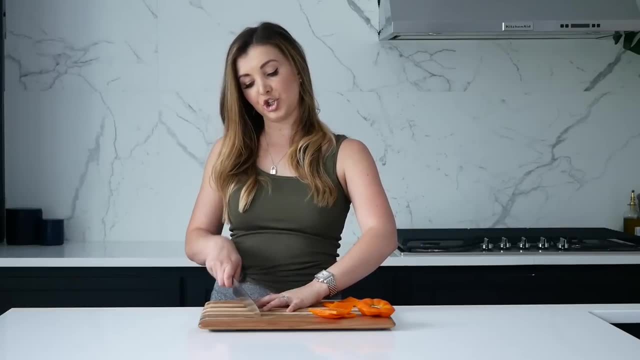 but they are. It's just not quite as obvious because they've learned over the years how to do it properly. So you want to grab things And the point of that is, if you have a flat hand and you're just pressing down the vegetable and you're chopping, what do you think is going to go? Your 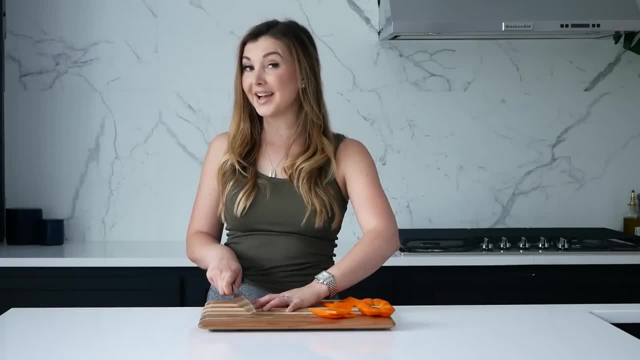 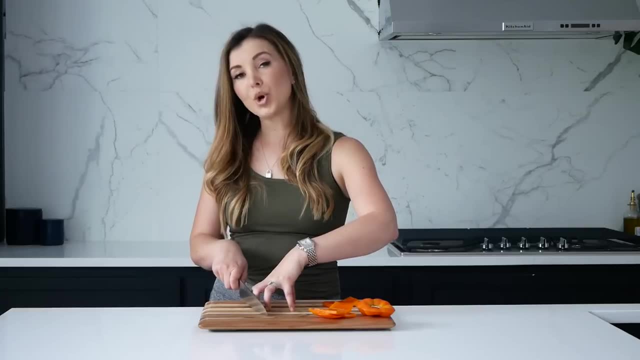 fingertip And trust me, it's not fun. It especially with a super sharp knife. it'll slice right through your tip and you'll have to go to the hospital. So if you have your hand in a claw form, the worst that's going to do. 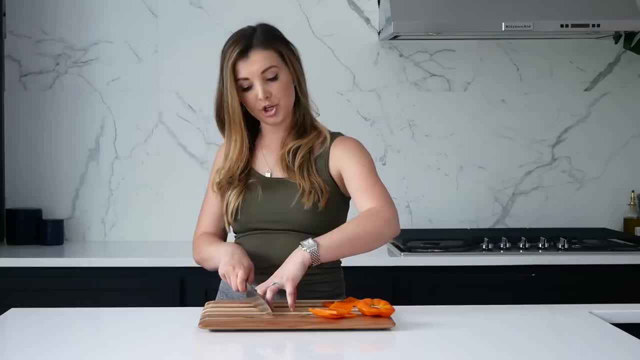 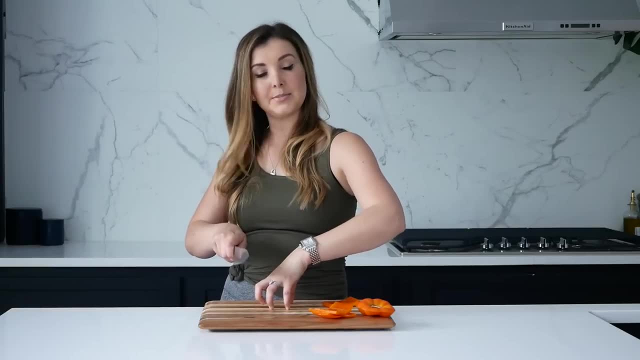 I mean, you literally can put your knife right up against your knuckle, which is actually what you're supposed to do, And if those tips are kind of curled under, you're not going to get to them. The worst thing that you're going to do is if your knife, kind of like, slips to side to side. 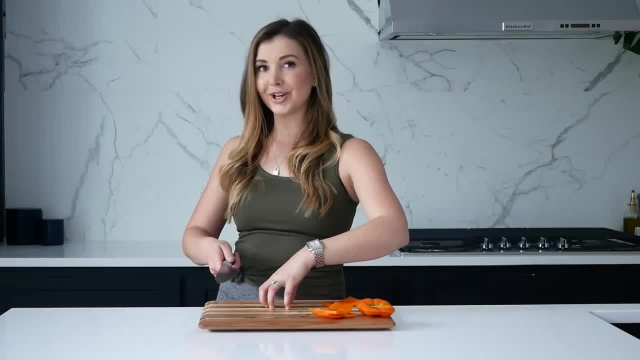 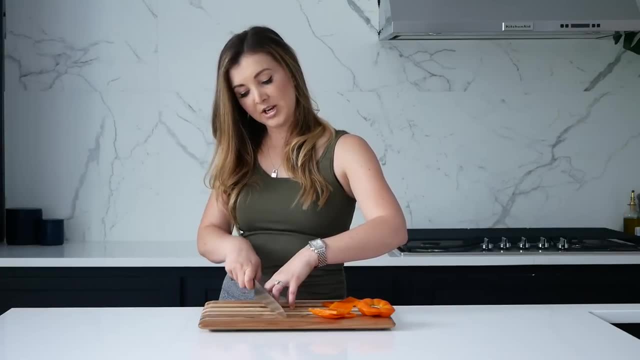 you might nick your knuckle- not fun, but not the end of the world. You're not going to go to the hospital because of it. So practice that a little bit. just practice kind of doing that boat rocking motion right up against your knuckles. I know it's kind of scary, but as long as you have, 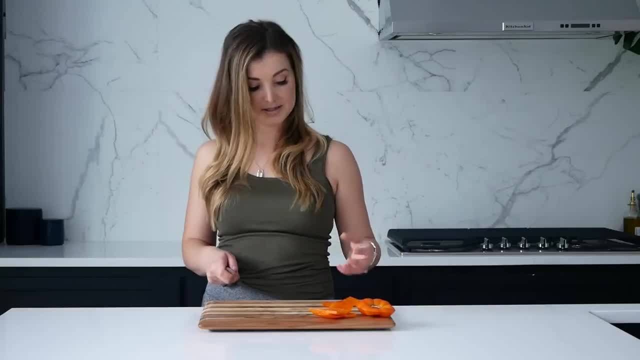 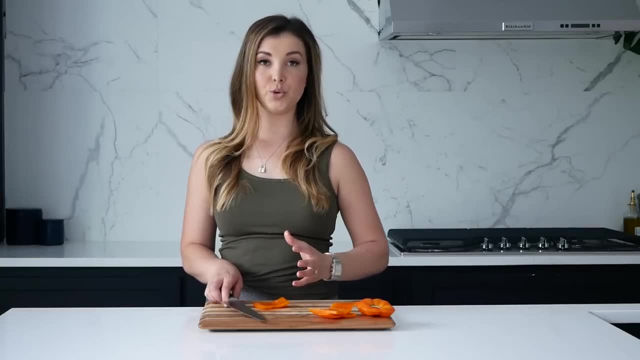 those tips, nice and hidden. you're not going to slice them, I promise. So first thing we're going to do is just slice this bell pepper. Everything that you want to do in cooking is: you want, when you dice or slice things, you want everything in uniform shape. So you don't want. 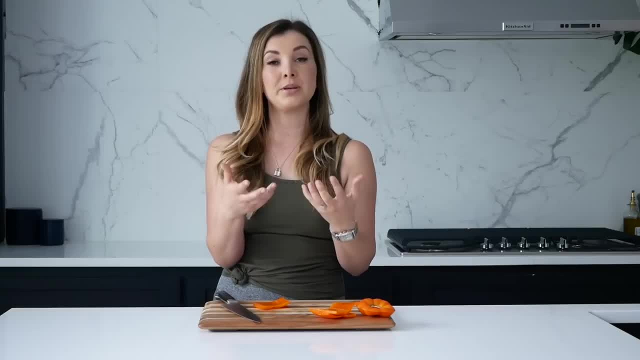 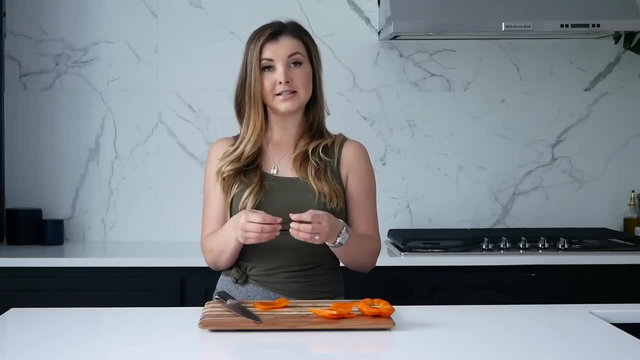 some slices this thick, some slices this thick, because then when you go to put them in the pan, they're going to cook very differently. So the idea of dicing things in a very similar shape and size is going to be all about having being able to cook evenly. So for here, 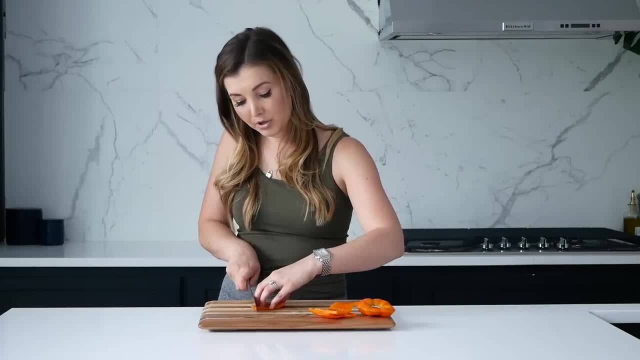 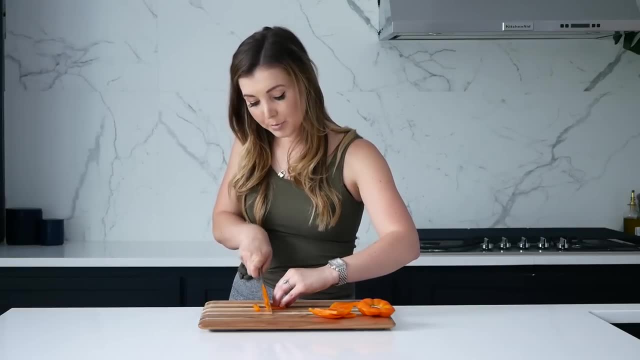 we're just going to slice. So get your fingers and you're going to do that rocking boat and you kind of try to make that same size each and every time. This takes practice And as you kind of pull back the knife, you're just going to go over slightly and then press down. 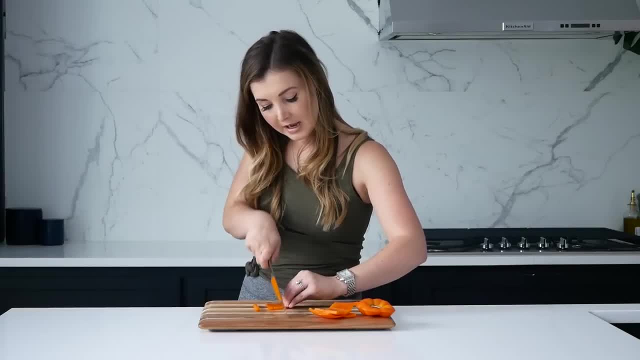 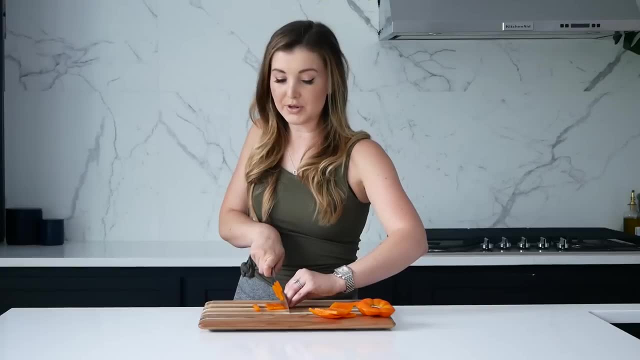 and just keep doing that, And that's how you actually now, if you get to this very end piece, people are a little scared to do it themselves. That's okay. You can either kind of put that in the compost, throw it in a salad later or, if you feel really brave again, tuck your fingertips as 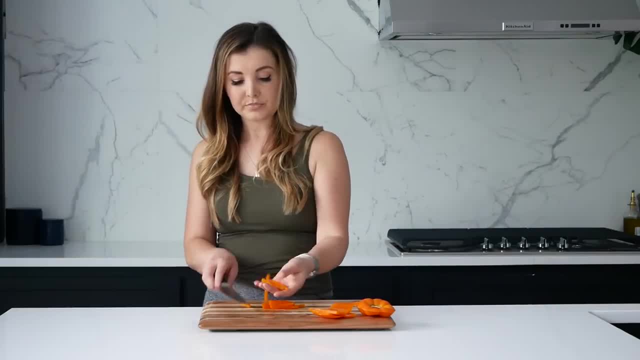 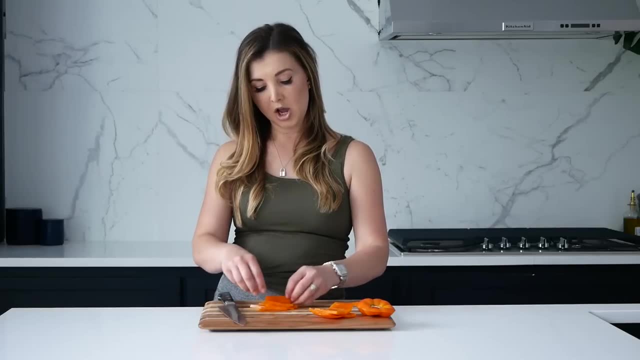 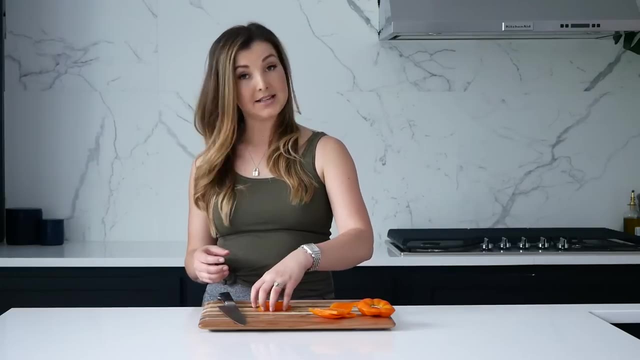 close as possible and then finish that last piece. So now you're going to see these nice beautiful little matchsticks. This is called a julienne. So julienne are just basically little matchsticks type pieces that you can do a julienne on really most any vegetable. So that is kind of how we're. 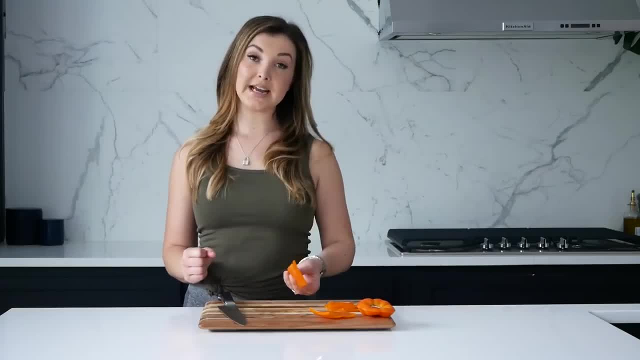 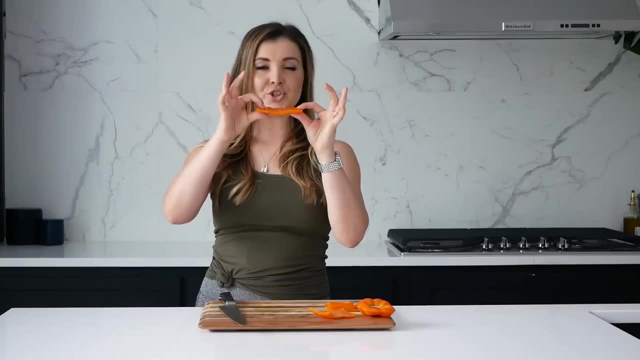 going to do those. We're going to move those to the side. Next thing, we're going to dice them. So whenever you want to look at, kind of, how thick your vegetable is, again with the bell pepper, it's kind of uneven. So it's not going to be absolutely. 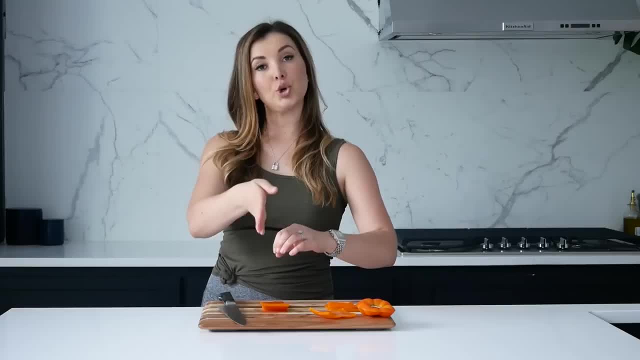 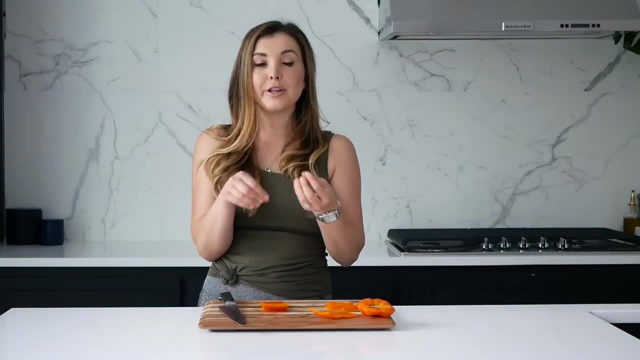 perfect every time, but you basically want to make your cuts the same width as the thickness of your vegetable And that's going to get those perfect, beautiful little squares Again. if you're not that concerned about it, you don't have to make it perfect, but that'll again aid in helping. 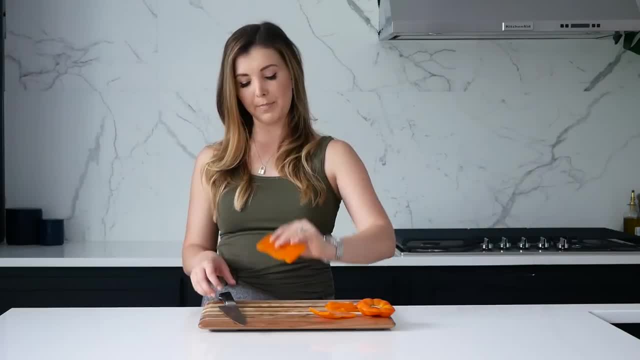 of everything cooked nice and even So, I'm looking at kind of how thick my pepper is And I'm going to go ahead and cut that into small pieces And then I'm going to cut it into small pieces And we are just going to make some long slices. So with here you can use that. 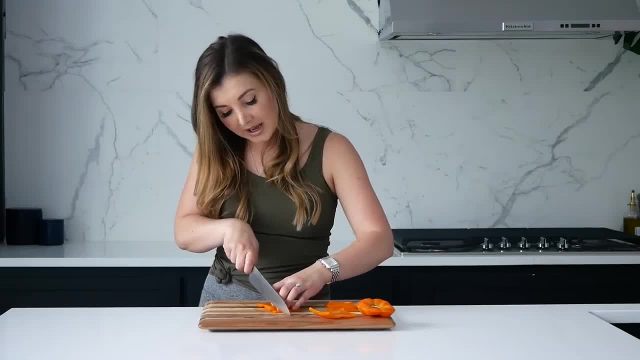 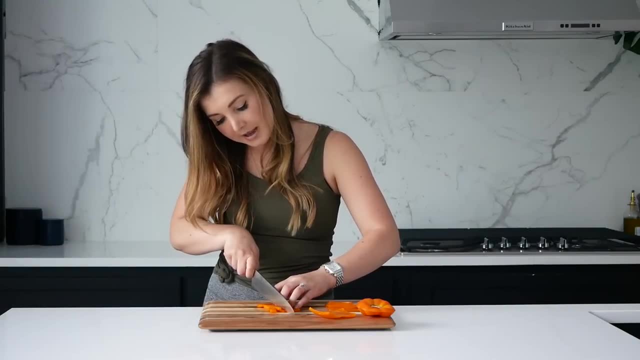 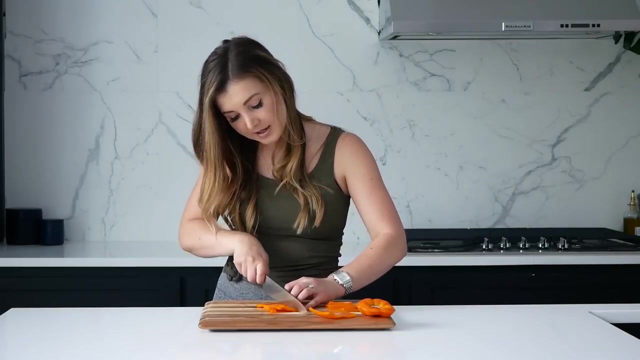 you'll always have to do the rocking motion. You can kind of gauge it with your eye, tuck those fingers and then kind of pull back And again use your eye. You're trying to make the same width of slices each and every time, And this is such great practice at home. To move, you can either 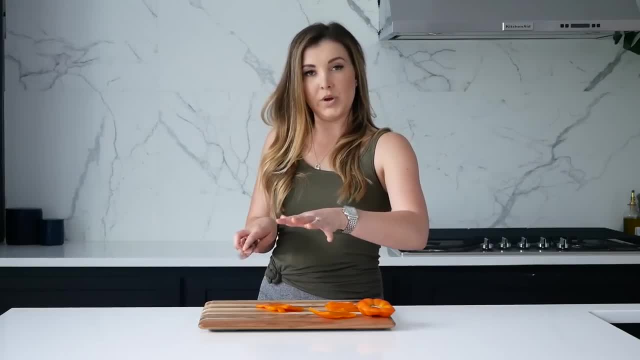 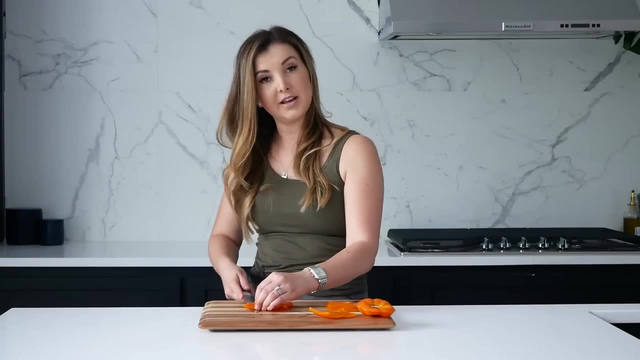 pick it up with your fingers, but sometimes all the little pieces you're going to have to wiggle on you. So another trick is get your knife super flat. just slide it underneath like that and then kind of move it with your knife And look at them, They stayed all nice. 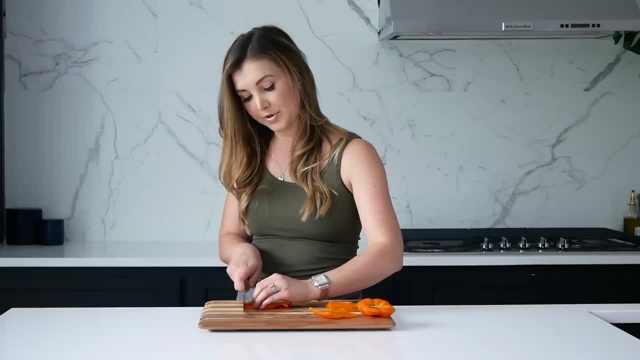 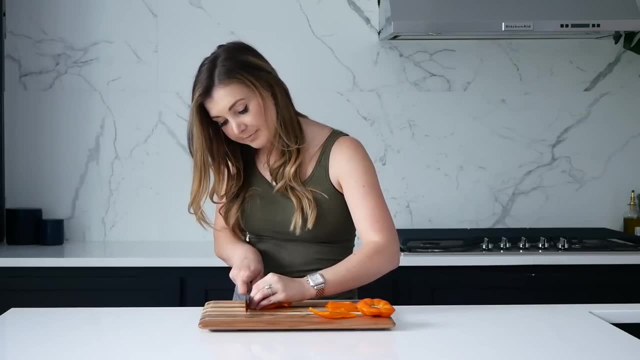 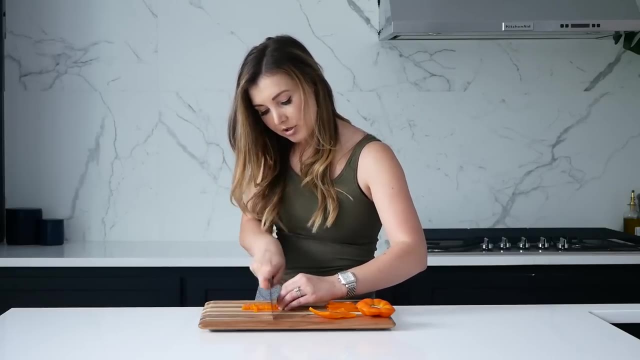 together and beautiful, And you kind of even them out with the tip of your knife. So now the same width that you want. that way you're going to do again to make the little dices. So again, you're trying to just make the dice the same size. Now I'm making these pretty small just for the sake of 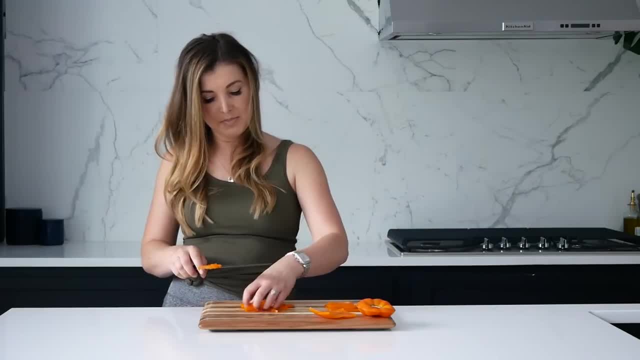 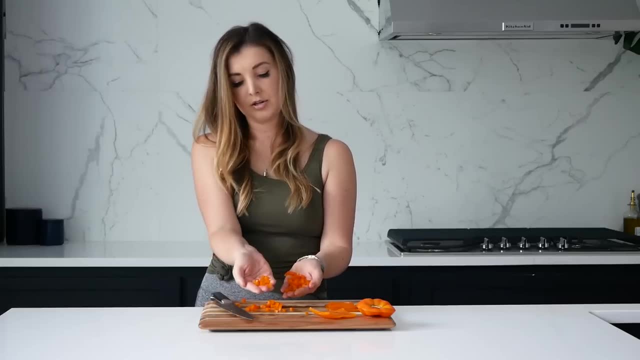 this video, but you can still use your knife if you want to. So I'm just going to go ahead and cut them. You can certainly make them bigger if you would like. So as you can see kind of all these different pieces in here, nice, beautiful small dice. So that is just a small dice of bell pepper. 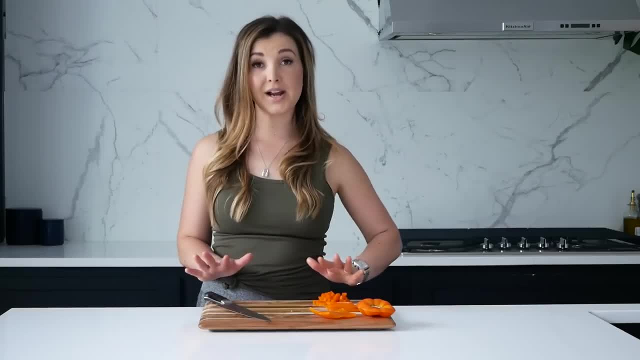 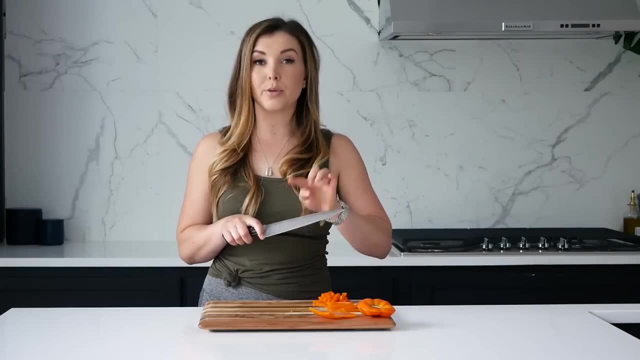 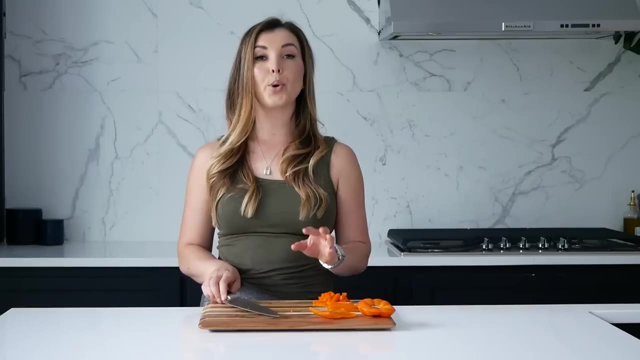 So those are two skills that I think you should definitely practice at home. So again, rewind. good knife fits in your hand well and sharp, sharp, sharp, sharp. It'll make your life a million times easier. It does not have to be expensive Vegetables. break them down to a manageable size. Make them the size 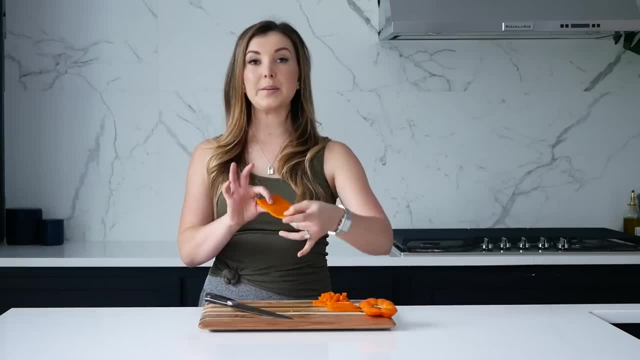 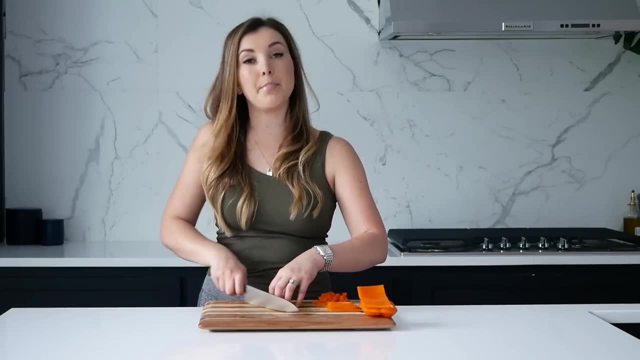 that you feel comfortable working with. So in this instance I did kind of three pieces like this: Slicing using that rocking motion, Practice, practice, practice. That's that boat kind of rocking motion. Get those knuckles up there with that bear claw Again. as time goes on you'll be able to relax the bear claw. 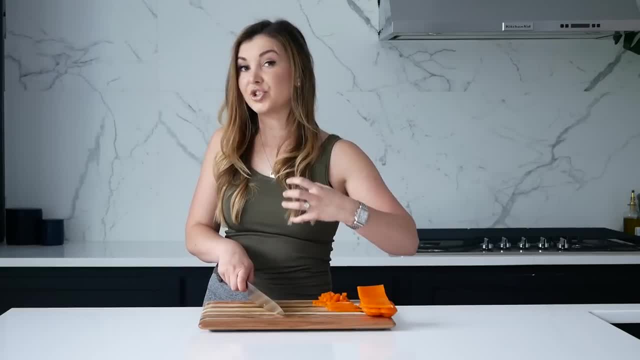 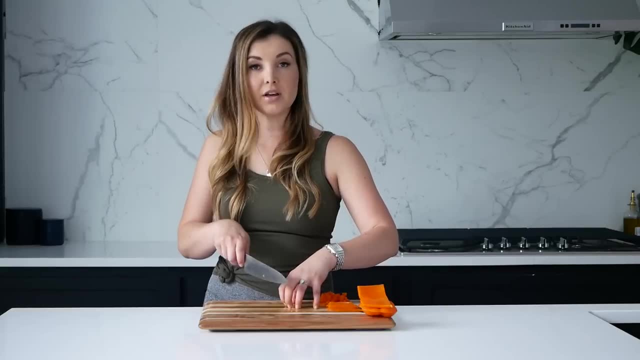 and you won't even realize you're doing it. It'll just come naturally. But that's what professional chefs do. I do it every single day. So again, practice that rocking motion. Practice it on vegetables. Practice your accuracy of the slices that you're doing and the 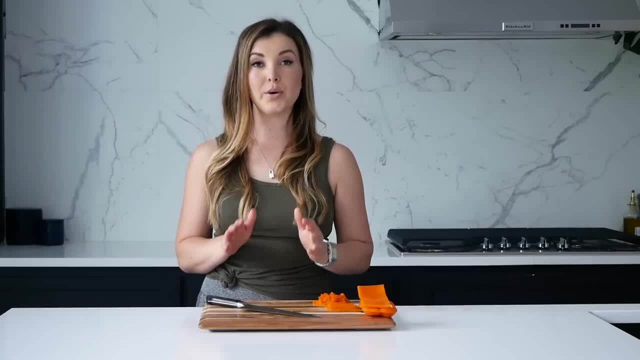 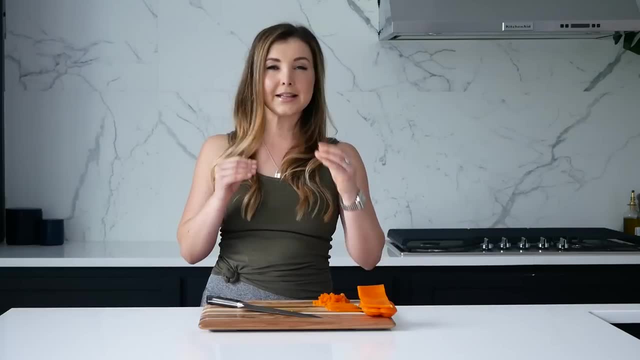 dices that you're doing. Key with dicing is you always want to make sure the strips and then the horizontals are the same size Every vegetable. you can't get to be exactly uniform in shape, That's okay, Don't worry about it.